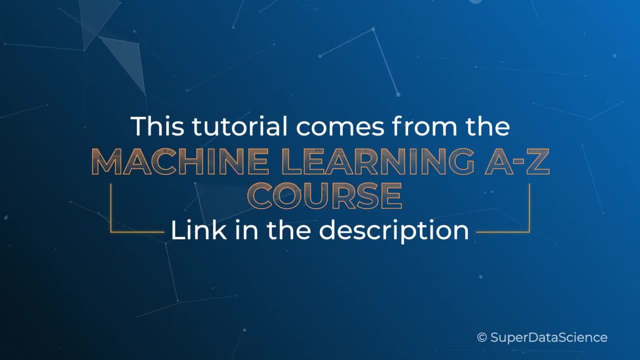 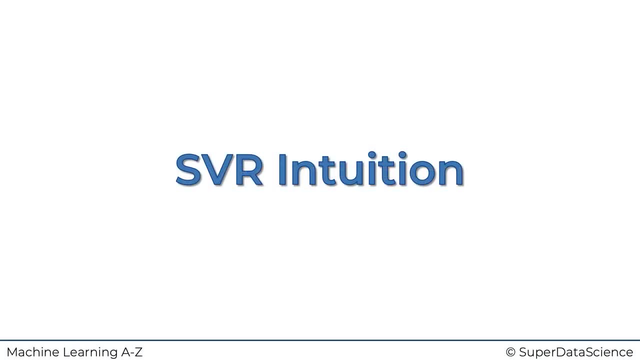 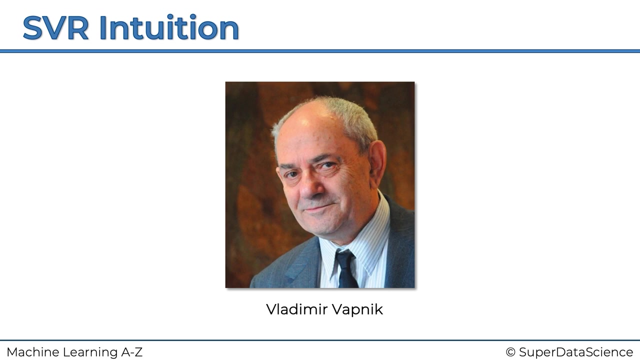 Welcome back to your machine learning A to Z course. Super excited to have you back on board. and today we're kicking off the support vector regression intuition. Super pumped about these tutorials, got some very exciting slides coming up for you. So what is support vector regression? Well, support vector regression was invented back in the 90s by Vladimir Vapnik and his colleagues who were working at the Bell Labs. at the time that was the AT&T Bell Labs, Now they're Nokia Bell Labs, And a lot of support vector machine and support vector regression are discussed in Vladimir Vapnik's book The Nature of Statistical Learning 1992.. 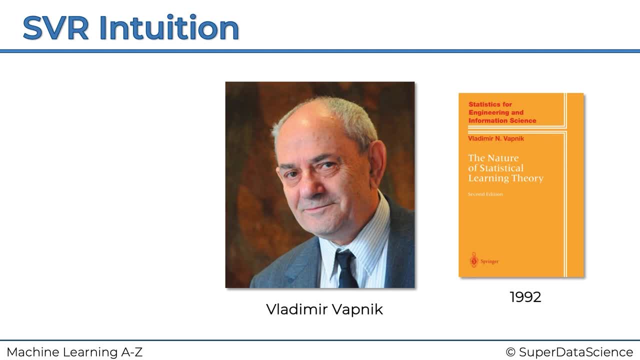 In this course we're going to talk about support vector regression. We will be covering both support vector machine in the part of the course to do of classification- and support vector regression. We'll be talking about it here And in addition to that we'll also be talking about kernel support vector machine and kernel support vector regression and the kernel trick and many other things like that. So there's a lot of exciting tutorials on these topics, But for now we're just going to limit ourselves to support vector regression, specifically linear support vector regression. 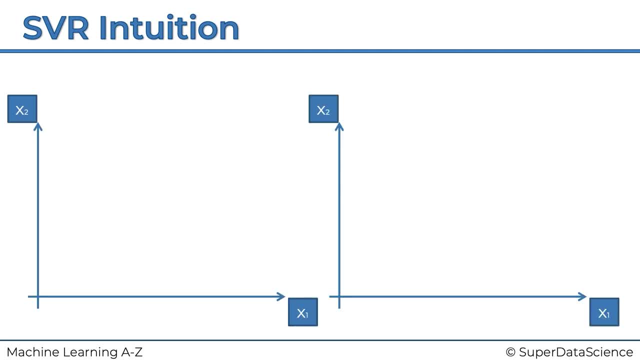 So here we go. Here we've got two plots And we need that in order to compare SVR to the simple linear regression. that will really help us understand things. So here on the left, we've got some random plots or random dots. I'm going to copy them over to the right So we know that these are identical. There's no tricks involved. There's a absolutely identical. This is an absolutely identical set of data, And let's start with the one on the left. we're going to apply a simple linear regression. We've already discussed what it's. 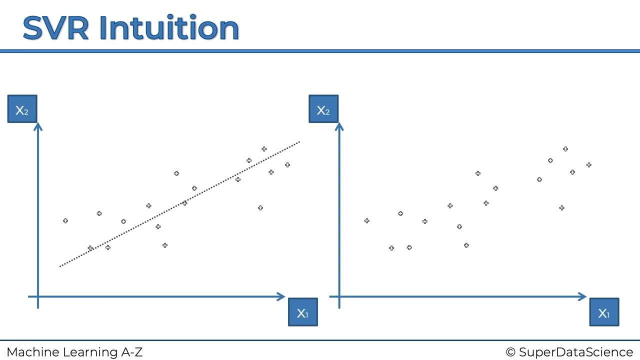 like, but let's quickly refresh. So basically, we're going to have this line go through the data. And how is this line derived? Well, a method called the ordinary least squares method will be applied to find this line. Basically, we want to minimize the distance between the- this value, y- the actual value in the data- and y hat, basically what it would have been on a trendline. we take the difference here, or difference here, we square it and we want to minimize that. that's ordinary least squares method. 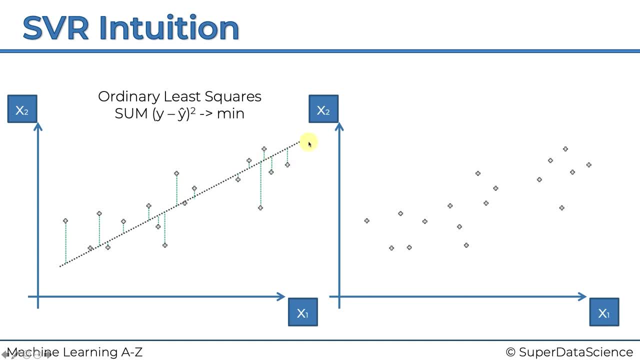 If, essentially, what we're doing is minimizing the error, we want to have a line with the minimum error possible. So that's, that's the intuition behind a simple linear regression, something we already talked about. Now, how does the support vector regression work? Well, let's have a look on the right With SVR. instead of a simple line, you'll see a tube, And here you have the regression line in the middle, but then there's this tube around. and what is this tube around? 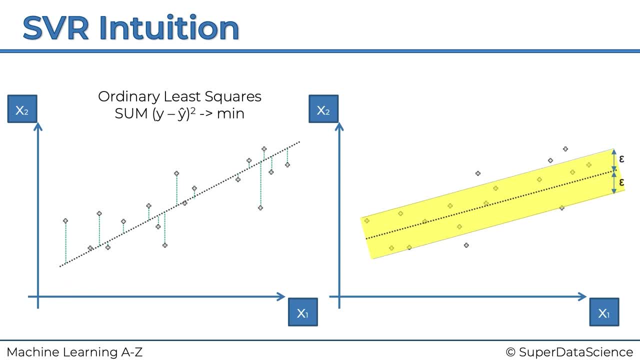 Well, this tube has a width of epsilon, and the width is measured vertically, is important along this axis, not perpendicular to the tube, but vertically. And this tube itself is called the epsilon insensitive tube. And what does that mean? Well, that means that any points in our data set that fall inside the tube they won't be will be disregarding the error. So, basically, this tube, think of it as a margin of error that we are. 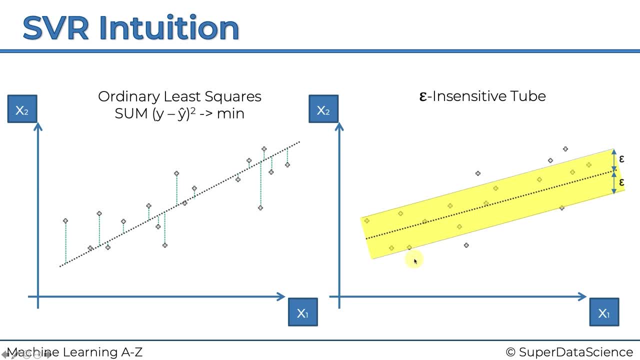 allowing our model to have and not care about any error inside here. So any discrepancy between, or any like distance between, this point over here and the line as in like, for instance here we could see- let's look at which point is that, that's 123.. This third point: you can see the line is even different. right, the results can be different and probably will be different. So this third point: here there's a distance between the line here and we care about this error here. we don't care about the error here. 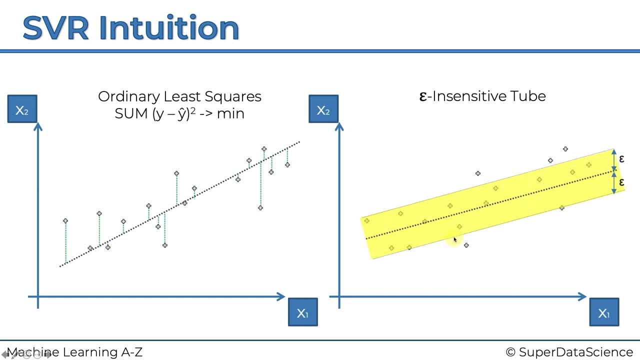 We don't care about this error because it falls within this epsilon insensitive tube. So we're disregarding any kind of errors in here And that's kind of the key behind support vector regression. it gives a little bit of movement or a little bit of buffer to our model And at the same time we have points that are outside the epsilon insensitive tube. There they are And for them we do care about the error, And here will be measured as the distance between 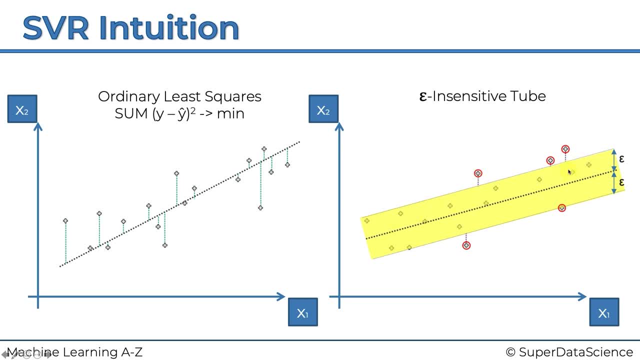 the point and the tube itself, So not the trendline but the tube itself. These distances have names. they're either xi star if the point is below the tube, or xi if the point is above the tube, And they're called so these values. xi are called slack variables. So it's either xi star if it's below, xi theta star if it's above. and we do care about the error. So we care about these distances And the way we care about it, so we're going to try to avoid 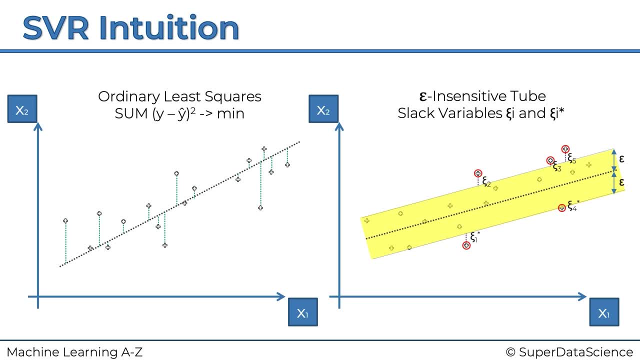 formulas. I will give additional reading, something you can look into further down at the end of this tutorial. But just for for completeness sake, here is the formula. So in the case of OLS it was a simple ordinary d squared like that. here is a bit more complex. We're not going to talk about this part over here, But what we're focusing on is this, and we can see that we're minimizing. we want these distances, the sum of these distances, to be minimal. 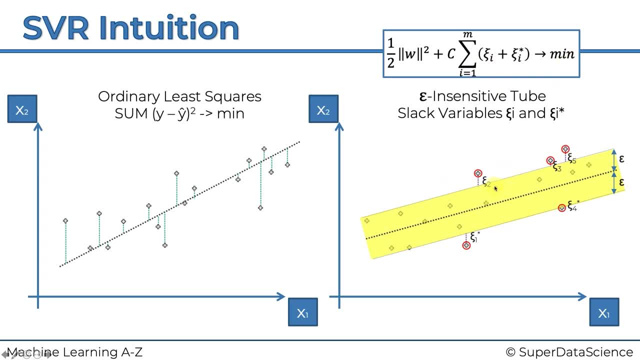 Once again, there'll be additional reading at the end if you'd like to go into it. But effectively these points, the ones that are outside our tube, are dictating what the tube will look like, how the tube will be positioned. So the error within the tube is completely disregarded. We don't care about the error, unlike in the ordinary d squared. So we're giving some kind of buffer of flexibility to our tube, or like allowing it to accounting for some kind of error that we might. 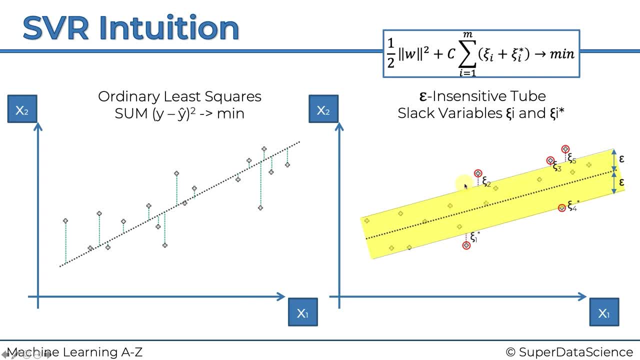 expect in the data. it's normal sometimes for there to be error, But these ones, they are important to us. And also one final thing: why is this method called support vector regression? Well, because effectively, these points, all of these points outside, but any point, actually any point on this plot is a vector right can be represented as a vector in this two dimensional space, or a multi dimensional space if you have more features. So in this case it's kind of presented by a two dimensional vector.